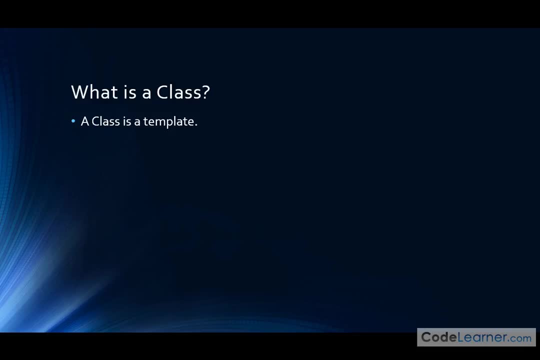 It's organizing a listing of logical characteristics that all of the actual objects that you're creating have to follow the template. That's what a template is. So anytime you read a book on Java And it says a class talking about this is a class, that's a class. this is a class, whatever. 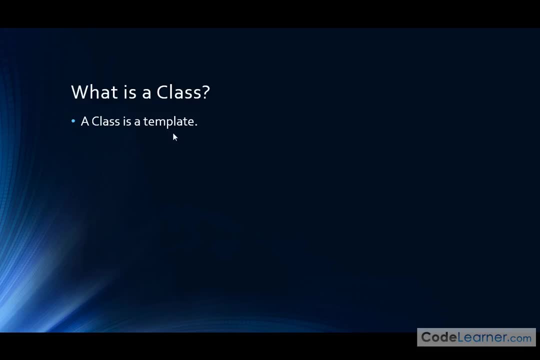 You need to replace this word with the word template. It's a really good descriptive word. Okay, a class defines the form of an object. That's all I'm basically doing is restating the first bullet. It's a template that defines the form of an object, just like we just discussed a minute ago. 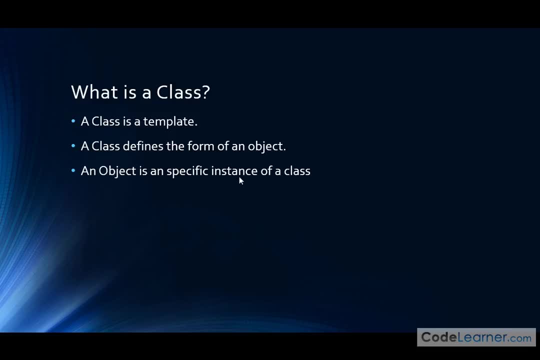 And here's the kicker: An object is a specific instance of a class. It's a specific instance of a class, So it's just the same. You know relationship that you might have already guessed. When you have a template, you define what something's supposed to look like. 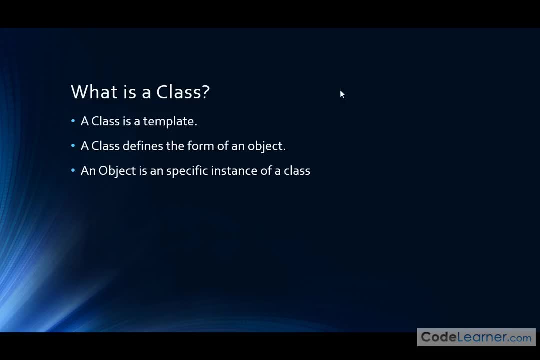 And then if you want to make copies or different types of objects, then you would just follow the template. Your different objects over here can look a little bit different, but they all have to kind of follow the same logical format of the template. So when we create an object in Java or any programming language, we're basically using the template to create a new object with similar characteristics. that's all spelled out in the template. 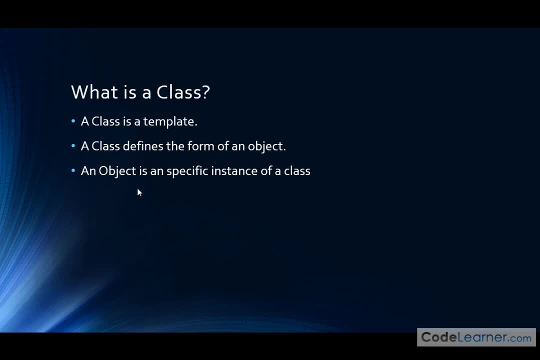 So let me give you a rock solid example. You know, talking about bullet points is nice, but an example really can get the point home. So let's give an example of a class and an object. Again, a class is the template and an object is what you create from the template. 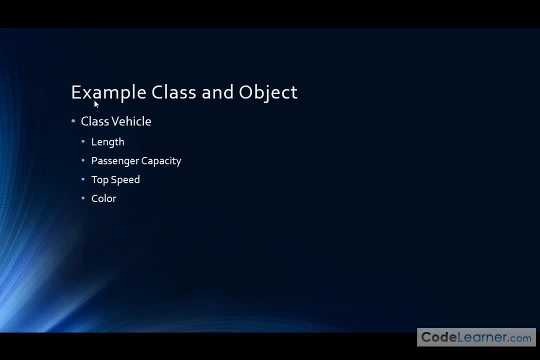 All right, following the template. So here's the best class that anyone can probably come up with. Here's a class of something we're going to call a vehicle. You guys know what vehicles are. Those are the things you drive on roads. 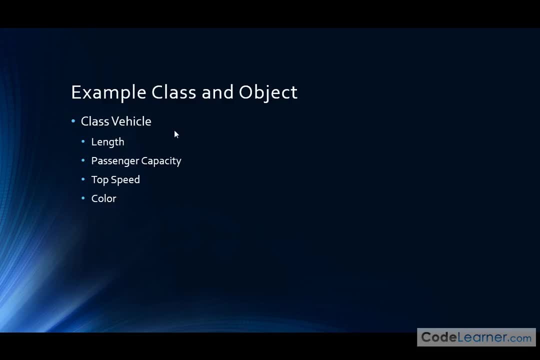 Some of them are big, Some of them are small, Some of them are fast, Some of them are slow, Some of them are 18 wheelers, But anyway they're all vehicles, So they share in common a kind of a function that we call vehicle. 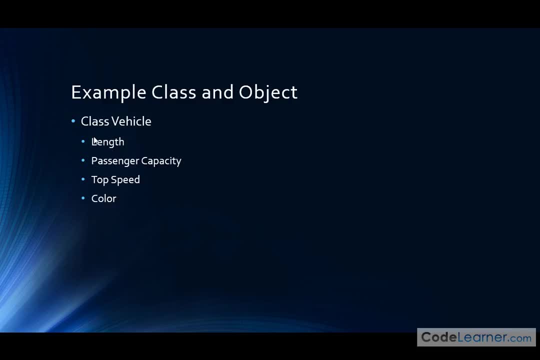 That's something with four wheels that we drive down the road right Now. there are many characteristics of a vehicle that you could write down. I've only written four here. Certainly we could say that all vehicles have some length, All vehicles have some passenger capacity that can carry five people or four people, or ten people or whatever. 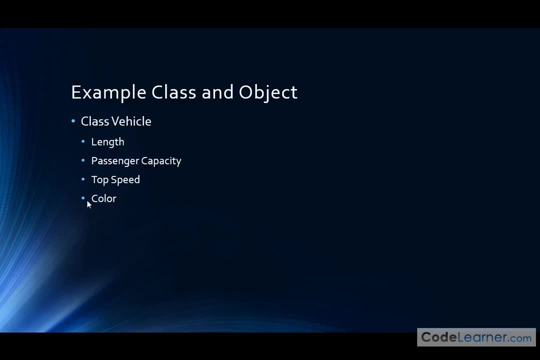 All vehicles have some top speed that you could look up in a book or on the web. All vehicles have a color, And I just stopped here. But there's many, many things you could define. You could say: what is the fuel efficiency of a car? 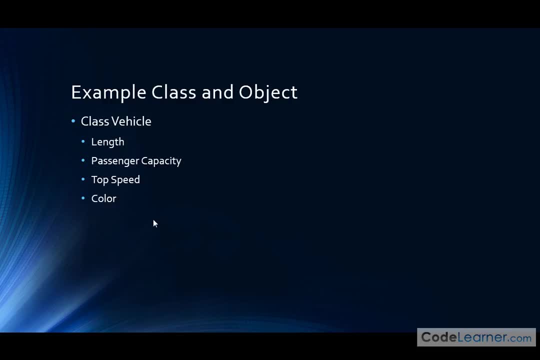 What is the price of a car? What is the maintenance cost of a car? I mean of vehicles, And so all of the things that you would list inside of your class definition is basically general characteristics of what the class is trying to describe. 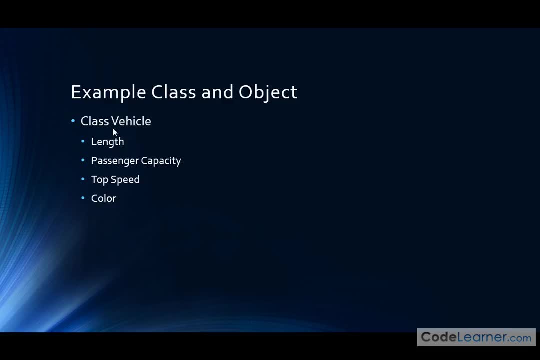 That's what a class is. It's defining this template here. This class that we're calling vehicle has to have all these characteristics, or whatever I decide to put in here. All right, And that's the template that I will then use to create objects which may have slightly different values for all of these things. 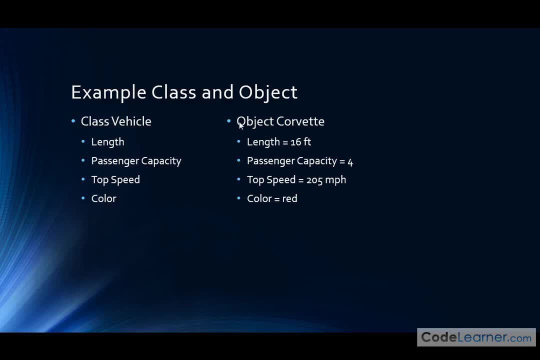 So, for instance, I may create an object. Notice, I'm not saying it's a class anymore, I'm saying it's an object and I'm going to call this object a Corvette. Now, a Corvette is a very specific instance of a vehicle. 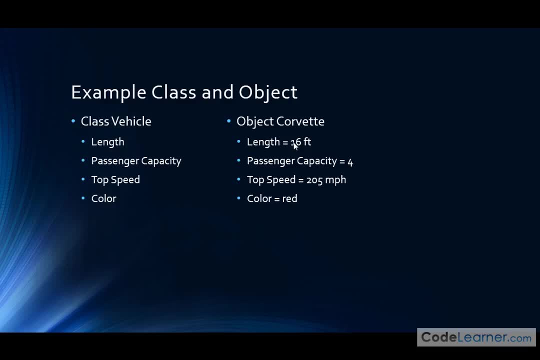 We all know what a Corvette looks like, really fast, sports car, right. We know that the length is a certain specific number. We know that the passenger capacity for this particular Corvette is a certain specific number. We know that the top speed for this particular Corvette is a certain specific number. 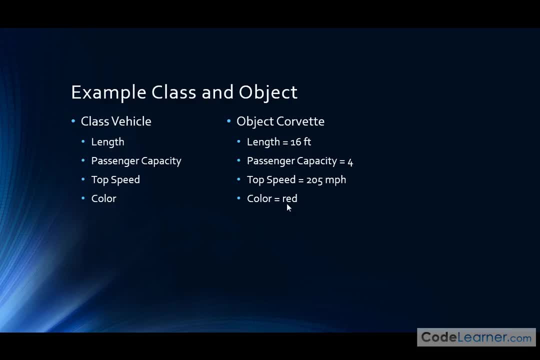 We know the color of this specific Corvette is a certain specific color, And if I had other characteristics in my template or my class, then I would have to have them listed when I create the object. Maybe I have fuel efficiency, Maybe I have cost. 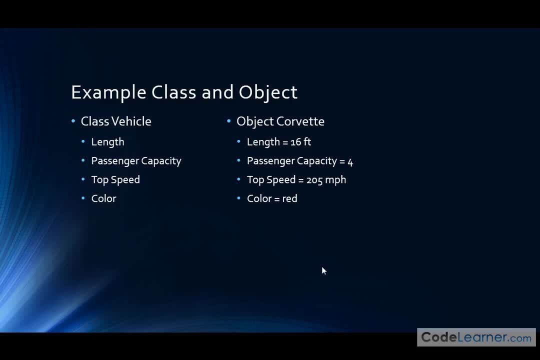 Maybe I have maintenance cost, Maybe I have, who knows, the size of the tires. Anyway, whatever you define in your class, which is a template, must be reflected when you create the object, because the object comes from the class. The object is created from the template called the class. Now let's look at 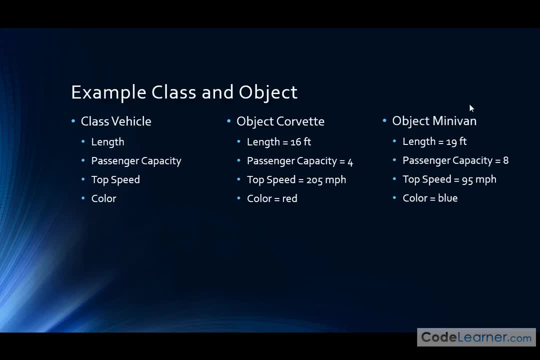 another object. This one's called object minivan. So here's a minivan. It has a length that's 19 feet. It has a much higher passenger capacity, It has a much lower top speed And it has this particular object. the one that I'm thinking of in my mind has a certain color, But again, 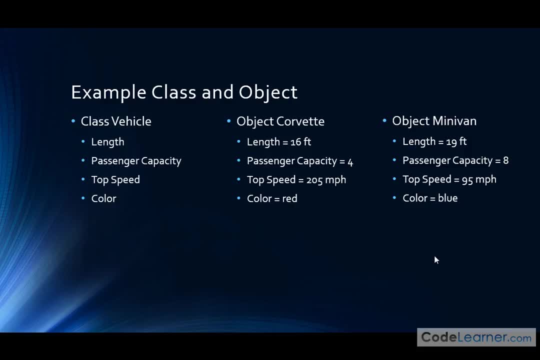 if I had other characteristics in my class, I would have to have them defined for this object. So now you can kind of sort of start to see why object-oriented programming is useful. Let's say I was writing a program that was dealing with cars. Maybe it's going to be a. 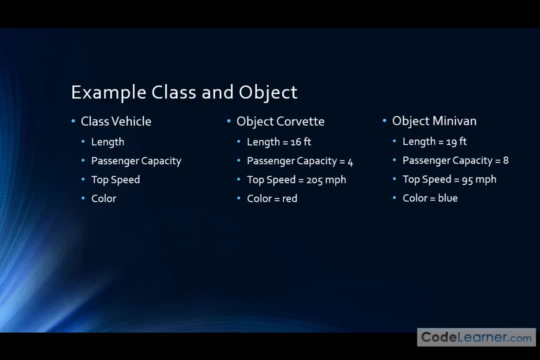 database of cars or a website or something that has a lot of car information. It would be kind of a pain to create a bunch of data structures for this car and a bunch of data structure for this car and so on, individually all the time, I mean when these things are so similar to one. 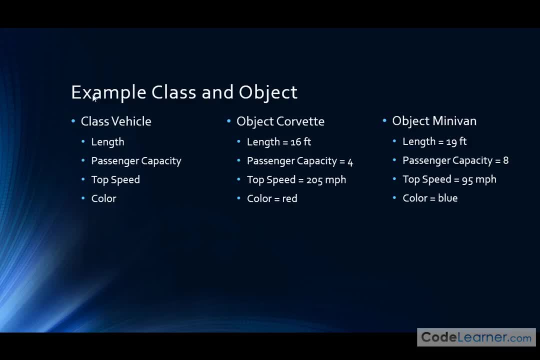 another. it makes more sense to define one central template That defines what the class is going to look like, And then from that I can create an object that we name Corvette, And then I can create another object that we name minivan. I might. 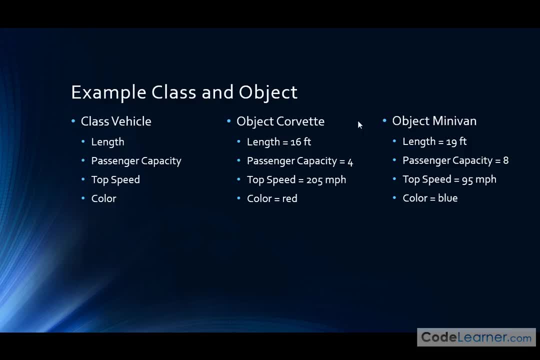 create a third object called pickup truck and a fourth object called Mazda 626 and another one that's called something else. So I can have as many objects as I want in my program, all created from the main template that's called a class. That's the major relationship between the two. 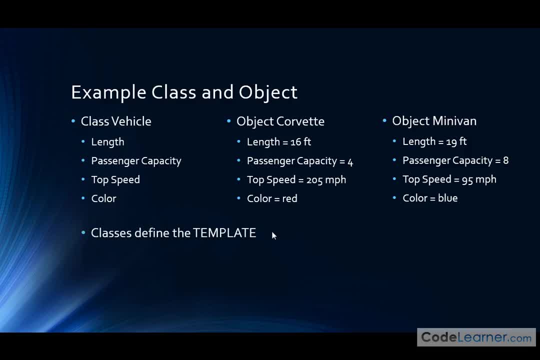 that I'm trying to drill in. So again, classes define the template. Objects are specific instances of the template. That's what you need to know. All right, That's the most important thing here. Now classes: in this particular example up here, we've defined values. You know, we said this class contains basically a. 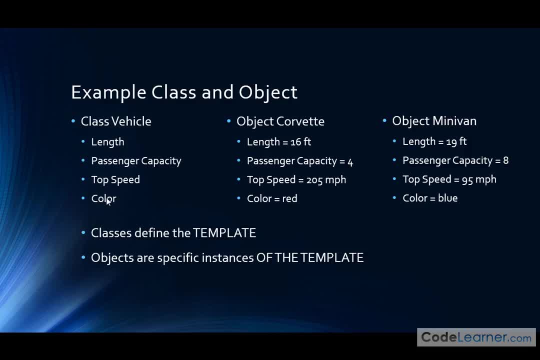 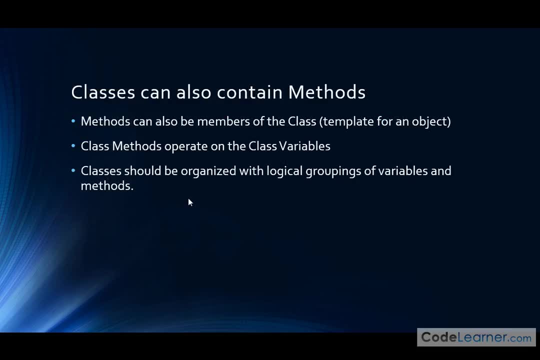 bunch of numbers: length, passengers, top speed. I guess this isn't really a number, but it's a characteristic, It's a data value. So far I've defined this class and I've said these are just data values, But in fact classes can also contain methods. So I'm going to define a class. that's. 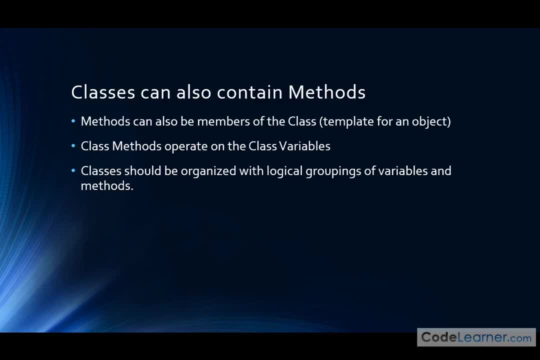 going to contain methods. Now. you know now why I introduced methods before. You should remember, a method is something that we usually use to calculate something in Java or perform a function in Java, But methods in the previous discussion that we've done have all been kind of these. 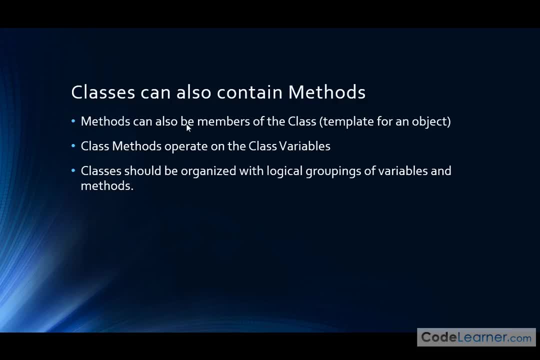 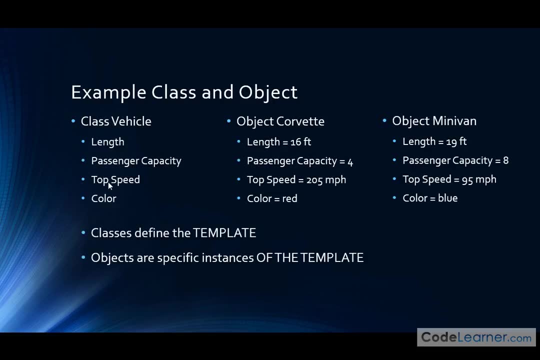 isolated things, But here we can add methods and they can also be members of the class. So we can have, for instance, this class template for vehicle. We can have this data, but we can also put a method in here that would be part of the class. So we can have, for instance, this class template. 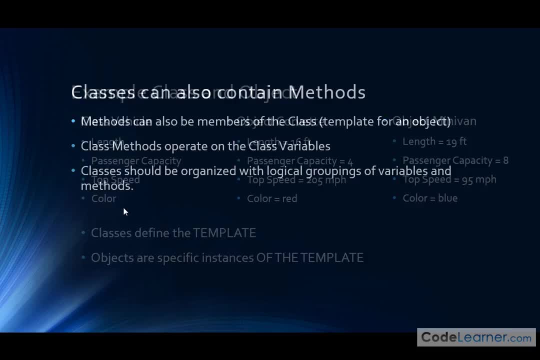 for vehicle. We can have this data, but we can also put a method in here that would be part of this class, depending on what we're trying to do. In general, when we create a class method like that, the purpose of them is to operate on the class variables, And classes should be. 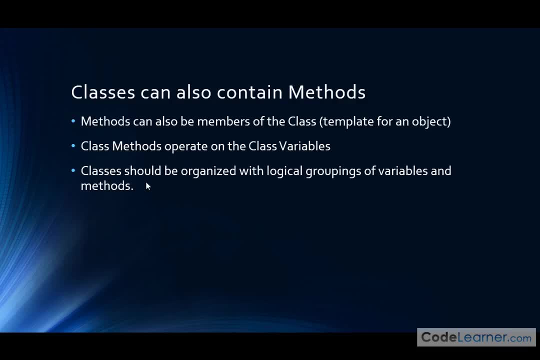 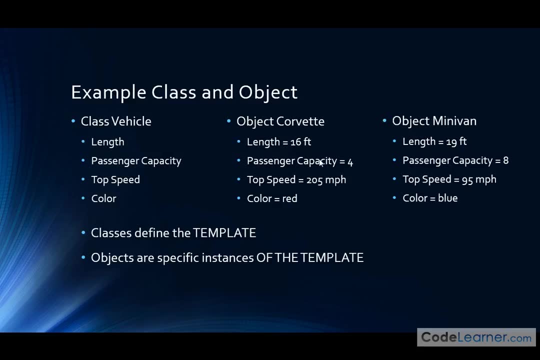 organized with logical groupings of variables and methods. What I mean by this- class methods usually operate on class variables- is here I have some information for the Corvette. you know the length, passenger capacity, top speed. I could put fuel efficiency, whatever I could create a. 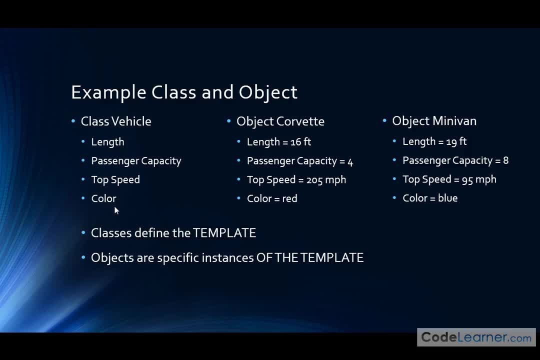 method here that would be part of this class definition. Maybe this is a method that would be. the purpose of this method is to calculate how long it takes this vehicle to go one mile. I could create a method Now that would be an actual calculation. I would calculate based on the top. 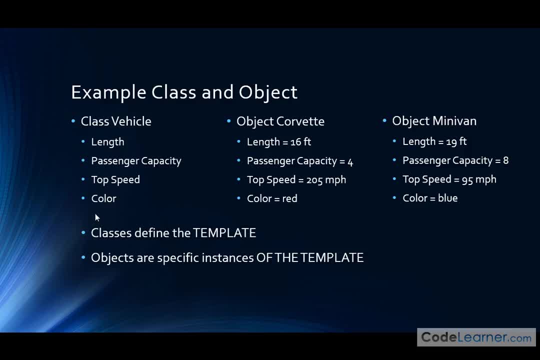 speed that I also have is defined as part of the class how long it would take to go one mile. Because if I know how fast it can go and I know the one mile, I can certainly calculate how long it would take. So I could put that in a method inside the class that would always be available. 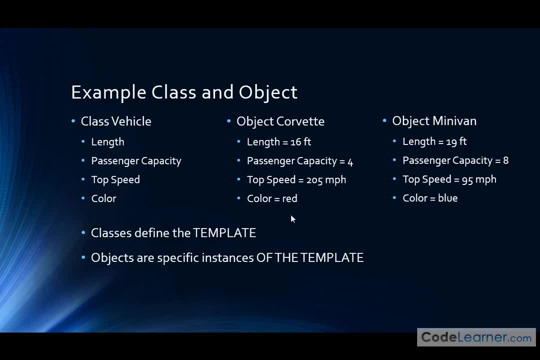 if I ever needed to calculate how long it took a Corvette to go a mile, It would always be in the in the definition, in case I always wanted to figure out how long it would take a minivan to go a mile. So I can define methods down here as part of the class that can. 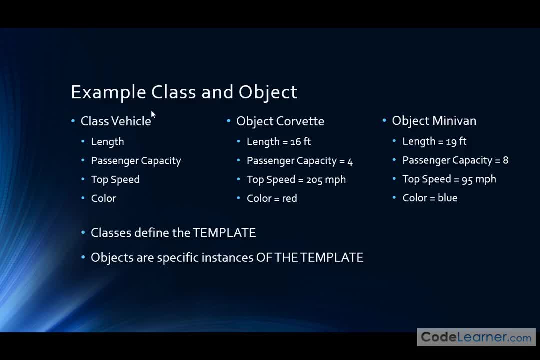 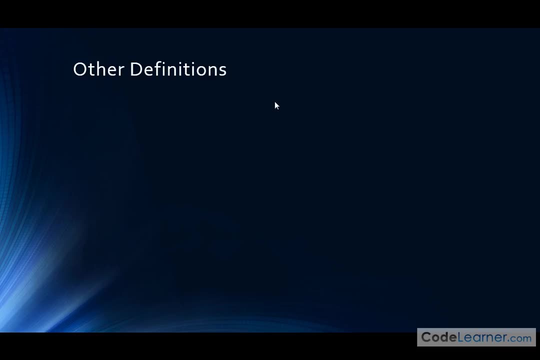 operate on these variables there. So when you talk about the idea of a class, you need to be thinking of variables that you can define as part of the class, right, and also methods that you can define that may operate on that information as part of the class. All right. so there's a couple of other. 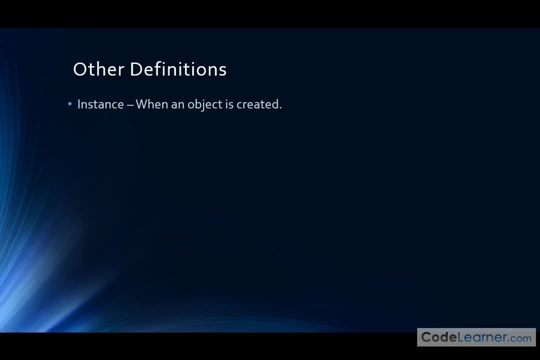 things that I want to talk about here. I don't want to go through them all at once, but I just want to point them out because you might read them in a book. if you're reading a book on Java, When you look at the word instance- I've actually used it a couple of times as well- 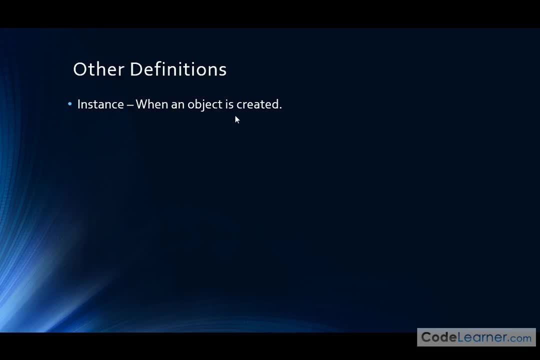 It's just talking about the idea of creating an object. See, when you talk about the class, nothing is really created with the class. The class is just the template, It's just the form of things. When you create an instance of an object, you're actually creating a copy. 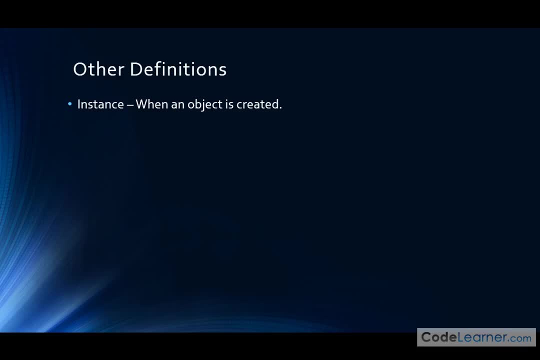 reserving memory, creating an object and you say that's a specific instance that follows the logical organization of the class. So when you see instance, you need to think about something that's been created. When you see the word member or class member, it just means the variables or 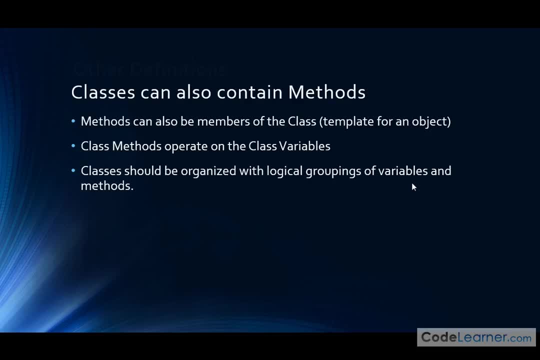 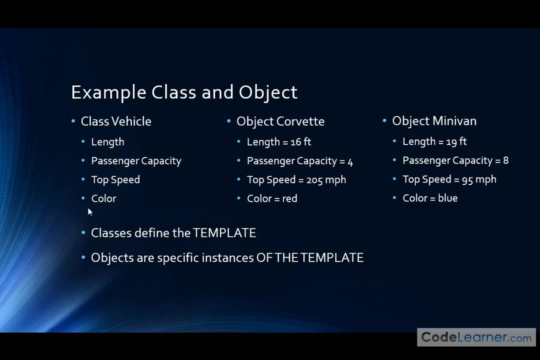 the methods that are part of the class. So up here, whenever I had this slide up above these variables up here, these are class members. If I had a method down here whose purpose was to operate on these guys, like we're talking about, that would be a class member as well. So it's just. 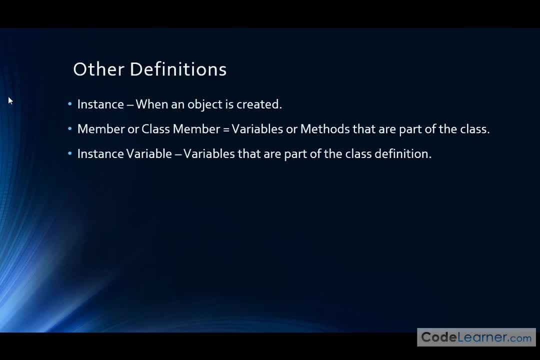 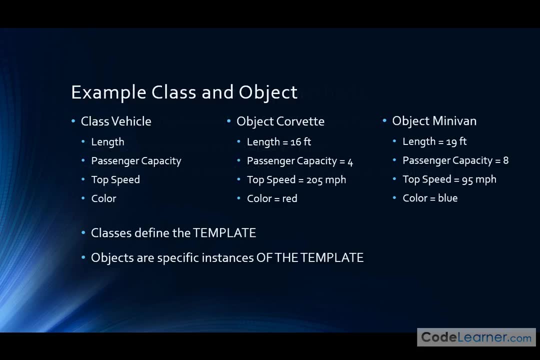 whatever is a member of the class, And also you might see something called instance variable. These are just the variables that are part of the class definition as well. So basically these same ones. here you might see these variables that are part of the class. You might see them listed as instance variables. These are just a. 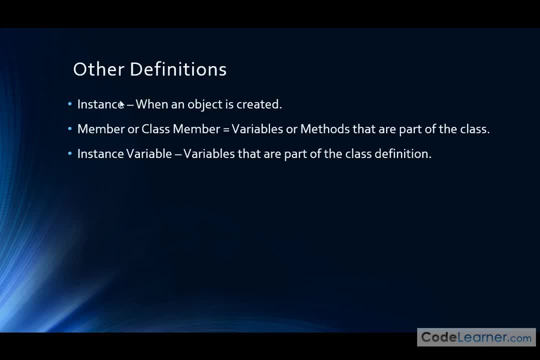 couple of different things you probably run into in a book. The most important thing is when you see the idea of instance. it's when something's created. A member is when you're looking at what consists, what does the class consist of? It consists of members, usually variables or methods. 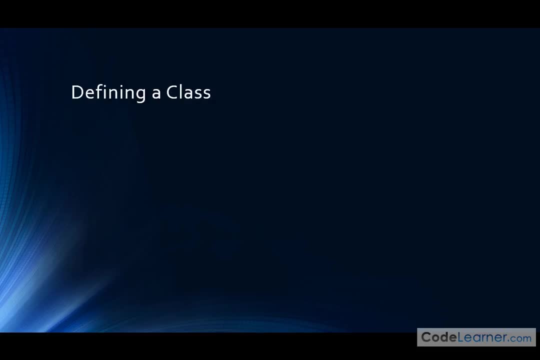 All right. so when we define a class- I'm not going to write code here, but I'm just going to give you a general idea- When you define a class, you use the class keyword and you have to give it a name And you. 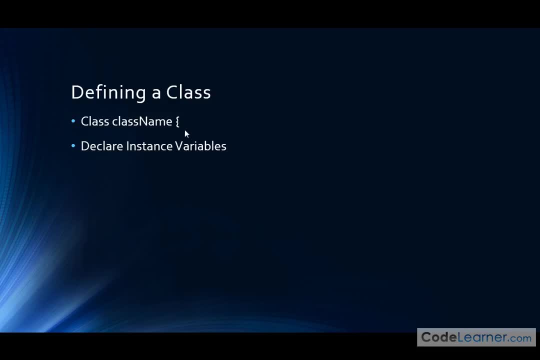 have an opening curly brace right And inside of this class definition, here you declare your instance variables. These would be things like top speed, color, whatever we were talking about in the previous slide. when it comes to the characteristics of the vehicle, That would be defined up here And you would 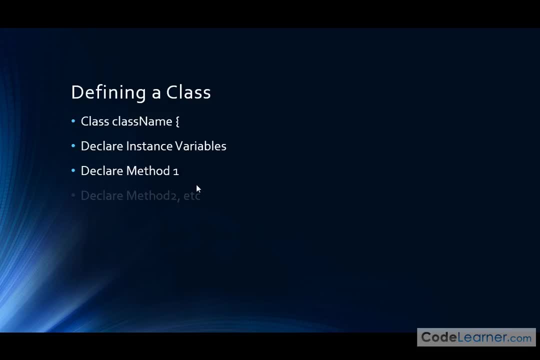 declare maybe a method here that would operate on these variables And you could create another method that would operate on these variables. You can have as many methods or variables that you want inside the class definition And then you have a closing curly brace like this. So when you define, 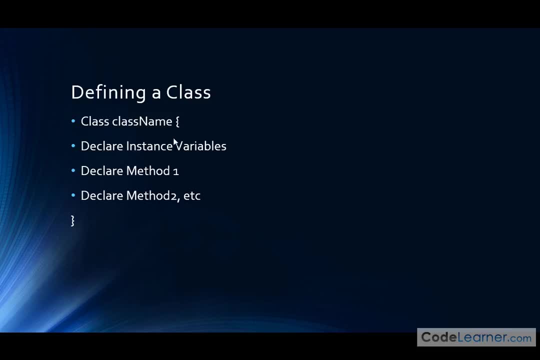 a class, you use the class keyword, class name, declare your variables, declare your methods, And that's really all I want to share with you in this particular lesson. It's so important. If there's one thing, just one thing, that I wanted you to take away from this lesson, I want you to. 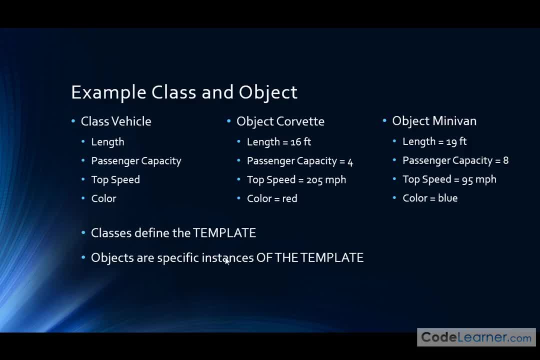 take away from this is that the class defines a template. Objects are specific instances of the template. You know, when you create and reserve something in memory of this form, that is called an object. So now, as you read Java books or learn about it more, or listen to me talk about it in the